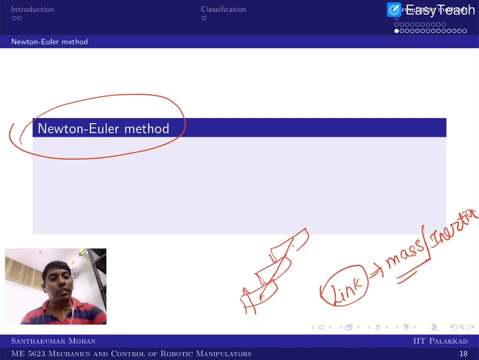 so first you have to actually like do the velocity propagation and the acceleration propagation forward, where we can start from the ground where the velocity and acceleration would be zero and we will actually like propagate based on the joints. so now, while we are going across what one can see- so for example, i am taking a nth link, so what i can see- there would be two joints and i 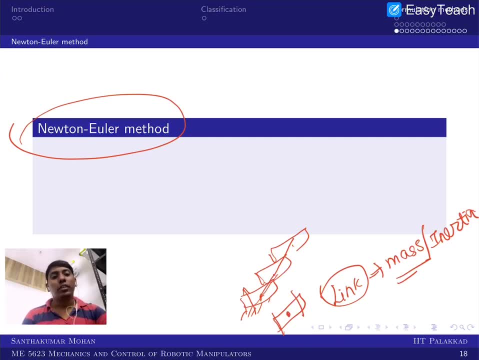 can see that there is a center of gravity, would be, you can say, possessed and that particular point, if it is actually like doing some action, or you can say it is actually like having a motion, there would be a resistance due to that motion. this is the motion direction i call. so then there. 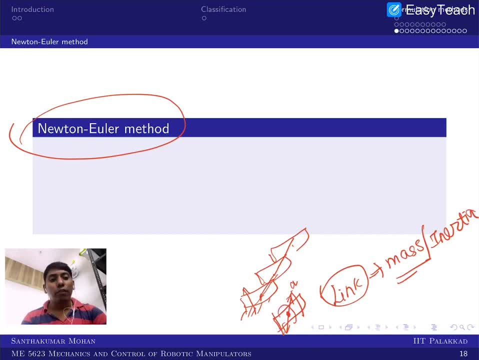 is the inertia would be opposing that. so then, in the sense, inertia, force and the moment would be acting on the centroid of the link. so in the sense, what we are going to do in the newton euler, we would be doing first joint, so the joint velocity and acceleration propagation. so in the sense, joint. 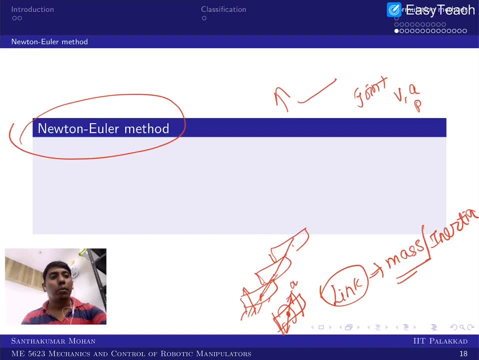 so i call velocity and acceleration propagation. okay, so the propagation is actually like what you call. uh, it is actually like forward propagation. so then, once each joint to joint, you gone, then the in between, the link, you call that the link- forces and moments you would consider. so this is also on the go of forward propagation. 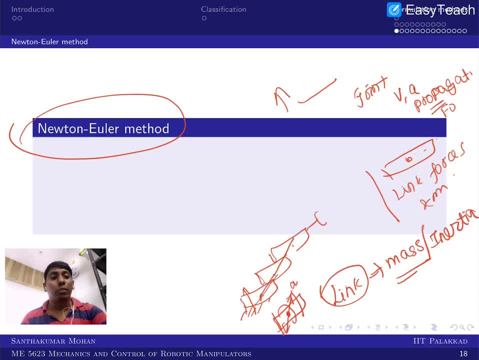 then what you can see, the end effector is actually a free link, because we are talking about serial chain and this point would be having a end effector force at the moment. so that would be known clearly. so then we can actually like come backward. so in the sense, so we will apply the static. 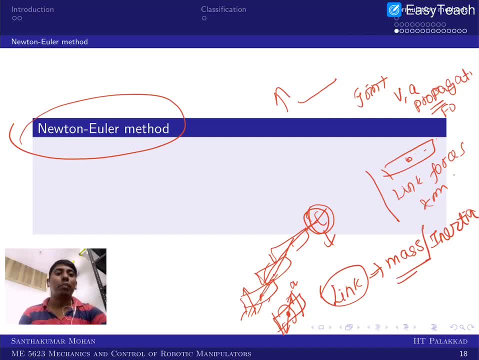 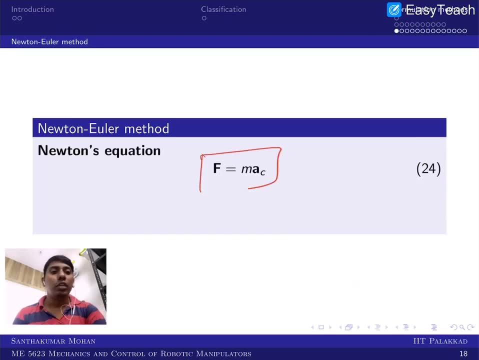 correlation, what you have seen, the sense here, we consider as a dynamic equilibrium and then we will come backward. so, in the sense, newton, euler method, although it is a simple but what, we are going to use the newton equation and as well as the euler axiom, we are going to use the euler equation and 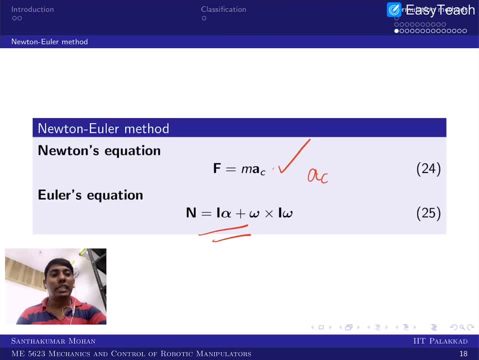 the newton equation we are going to use. so here, ac is not straightforward ac. so this is actually like what you call centroidal, uh acceleration. the centroidal acceleration, linear acceleration, that would be having several component. there is a slip acceleration, there would be a, you call. 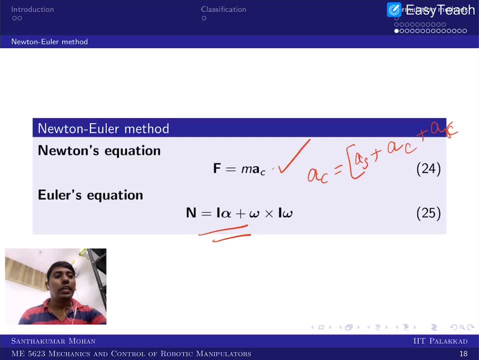 corollis acceleration, then there would be a centripetal or radial acceleration, then there would be a tangential acceleration like that. everything would be consistent. similarly, you can see here. so this is actually like going to give something like a gyroscopic effect and this is 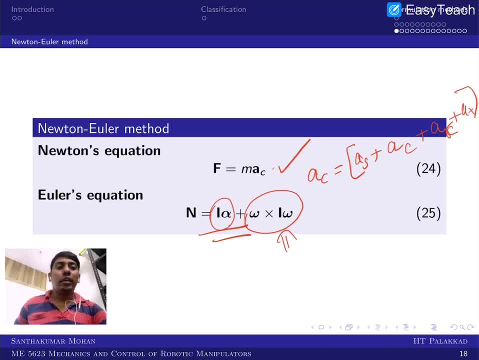 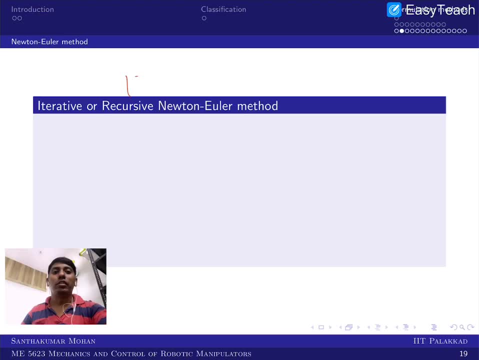 what you call the general, uh, you call angular momentum, right, so this is what the newton and euler equation we are trying to use. so now you, in the sense I told this is a recursive method or iterative method. we will start i equal to 0 and go n then. 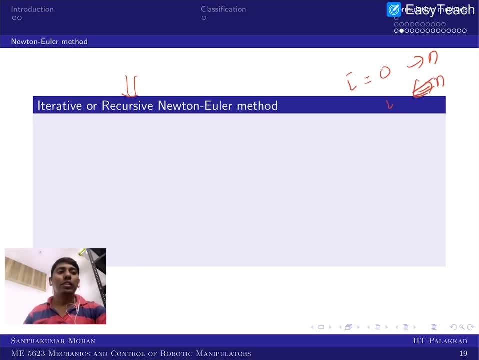 we will start from n. you can say backward 2, you can say 1 or i equal to actual, like n, we start and we will come back to 0. or you can say 1 based on what we are seeing. so you want base forces. you 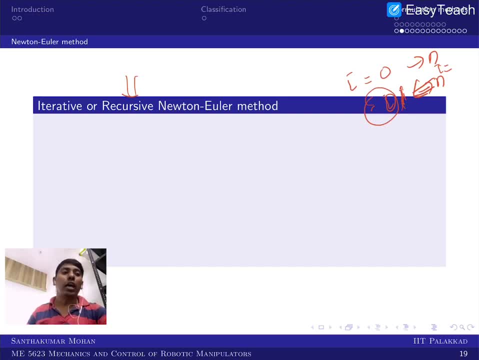 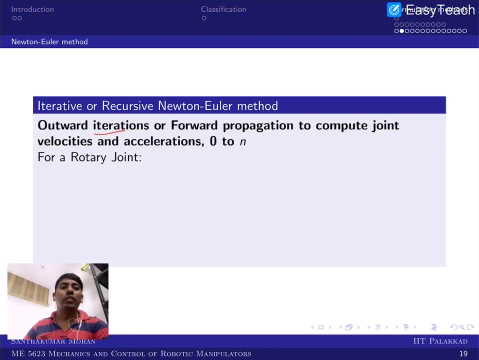 will come to 0. you want actually like only the first joint force and torque. then you can stop up to one. okay, so this is the way we are actually like starting. that's what I am saying. so we will actually say outward iteration or forward propagation, but to compute the joint velocity and acceleration. that is what we are trying to do. 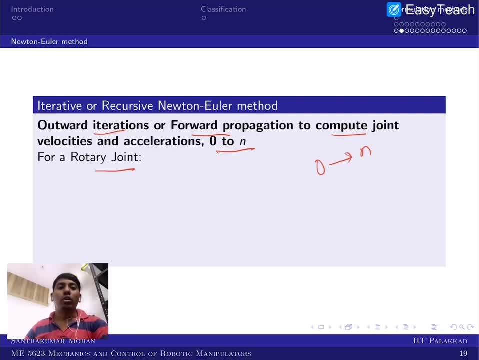 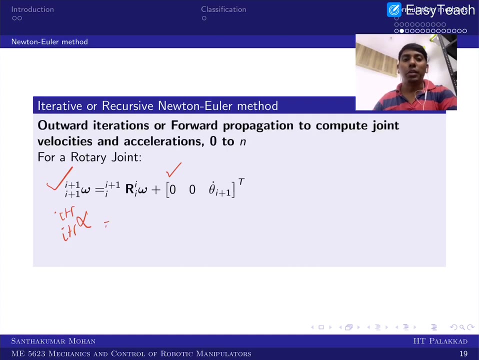 where you start from 0 to n, you go, for example, rotary joint, what would be the case? so we will say the velocity in the sense differential kinematics. we have done this, we will take, and similar way you can actually like, extend for the acceleration what you can see, alpha i plus 1 to i plus 1, that would 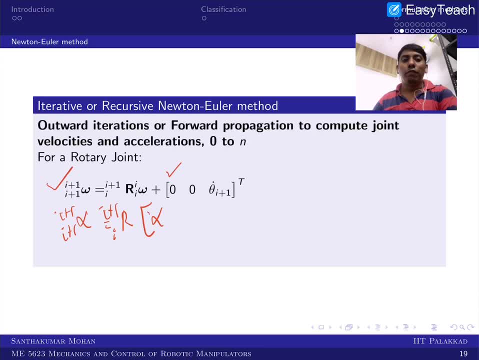 be r, i plus 1 to i, that would be alpha i to i. then what you will have? so you will have a cross thing. what cross thing that would be having. you can say additional cross to cross. and then you will have the second thing, which is actually like 0, 0 theta double dot of i plus 1. so that is what we. 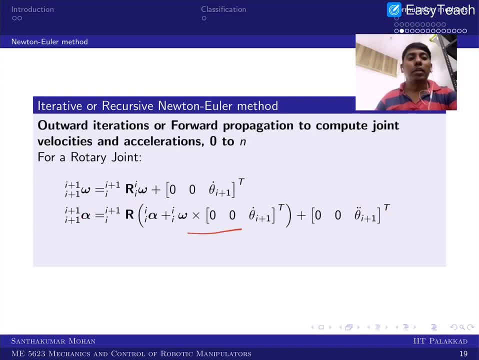 are actually like doing it. what? in the sense you have a gyroscopic moment where the previous joint angular velocity and the current joint angular velocity can be having a couple. so that can be accommodated here. so in the sense you can see that that can be taken care further. so in the sense, 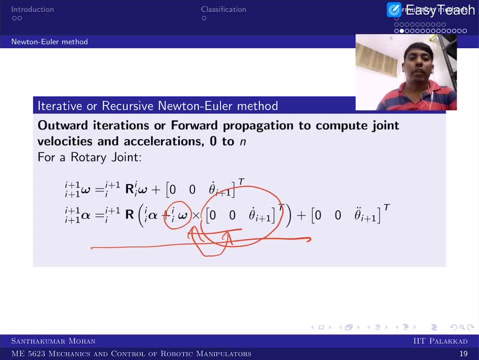 this is what we have done And this is the way we can actually like propagate for the angular velocity to the angular acceleration. now we will actually like get the linear acceleration because linear velocity is not really required, because alpha and omega is sufficient for finding the linear acceleration. 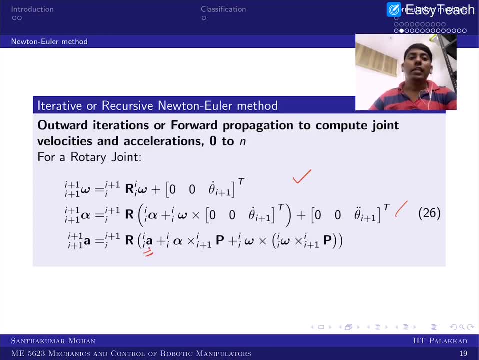 so in the sense linear acceleration also like a previous linear acceleration, and then you can see tangential acceleration, then the radial acceleration. if, if, if this is actually like you can see a presbyter joint, there would be a corollary and as well as slip will come right. now we are talking about the radial acceleration. So now you can see if it is a rotary joint. these are the three equations we are going to use for the forward propagation, for finding joint velocity and acceleration. but as a presbyter joint, what would be the case? so the same thing. you can see the presbyter joint, that theta 1, dot would not be coming. or you can say theta 1, theta dot, i plus 1 would not be coming. and similarly you can see that there would be a velocity. propagation is required because there would be a corollary component. so we are actually like taking the velocity and then we are talking about that. 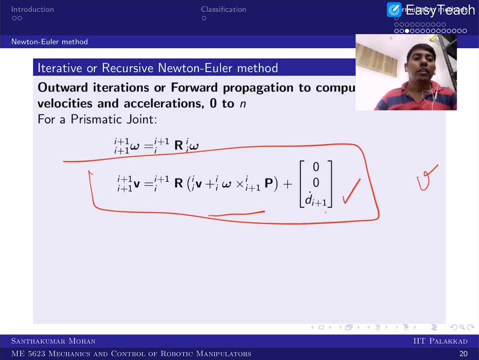 you can say propagation. So there you would be seeing that there is a slip velocity is coming in this. So then, further, you are taking the alpha i plus 1. with respect to i plus 1, there would be no. you call theta. you can say 0, 0, theta, double dot i plus 1, because that is going to be 0 in. 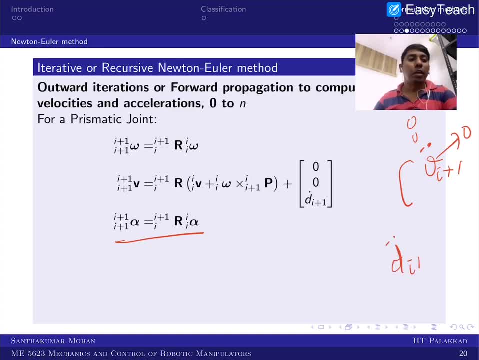 the prismatic joint, whereas you would have d double dot, i plus 1 be there. So then, what we are seeing, so you can see that this is the previous, you can say, joint aspect, but this is the current, and the current angular velocity and current linear acceleration would be having a 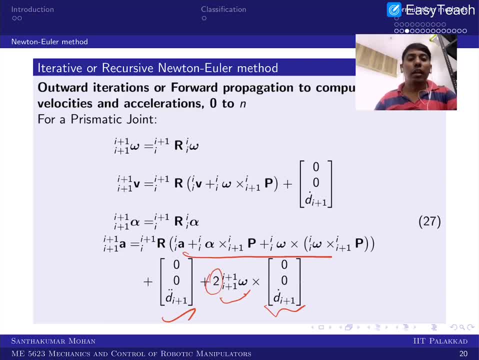 you can say Coriolis component, You can see that that is a two times and this is actually slip acceleration. this is a Coriolis acceleration, this is a radial acceleration, this is a tangential and this is the previous joint acceleration, right? So these all actually like accommodate. now what? 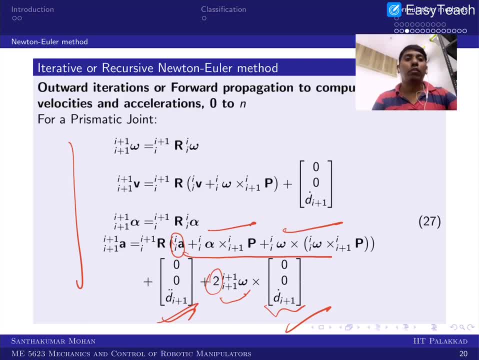 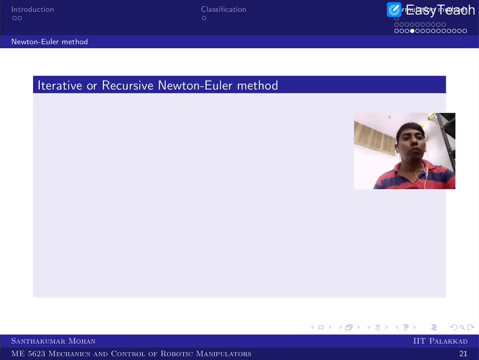 we have done. we have done the outward iteration, which is forward propagation you call either it is a rotary or prismatic joint. we can definitely get the joint velocity and acceleration. Now we will move forward. So what we can do, we know now joint velocity and acceleration. what we can do, we can actually like. 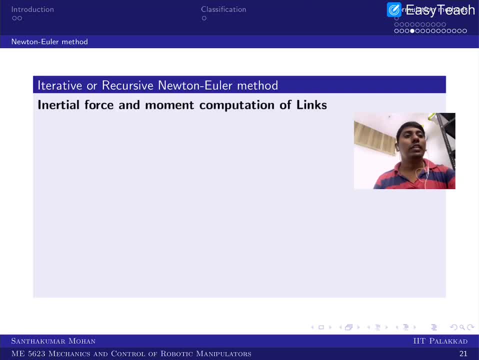 find the link force and link moment. So, in the sense, link inertial force and link moment we are trying to find. So, in the sense I am writing, that is actually like f, which is nothing but what we are trying to do: the link mass we are considering and the center of you can say centroidal. 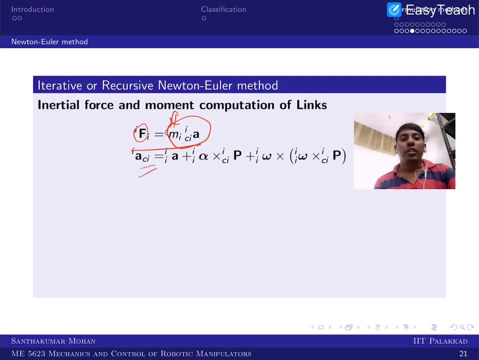 acceleration we are trying to calculate and what you know, the inertial force would be opposite to that. So, in the sense, f equal to m a c. So that is what we are trying to do. So we are trying to substitute and we are trying to get the- you can say- link force. similarly, the link moment also we can. 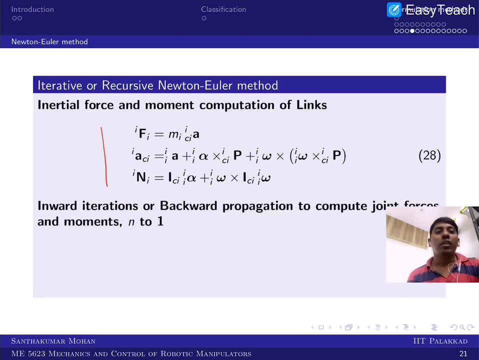 calculate and we can actually like get. that is what you call forward- propagation of the link forces and link moments. So now what you can do, the next case, you know the Nth joint. you can say end of factor forces and moment and you are come in backward. So in the sense, these are the link. 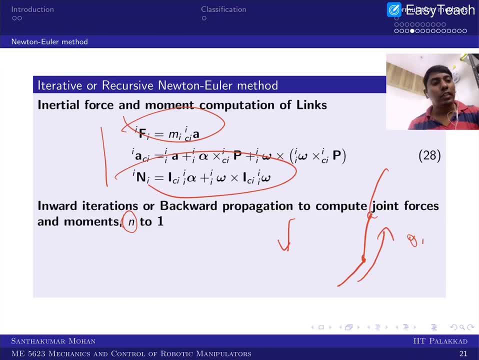 So what you are doing, the forward propagation, you are calculating theta, theta, dot in the sense I will call so you can see that what we are trying to do. so we are trying to find out the q dot and q double dot aspect and while we are actually like coming return, so we are actually like seeing that the 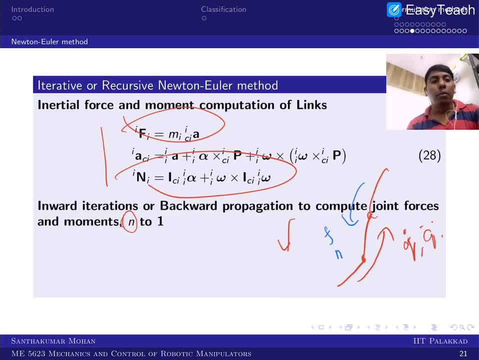 end effect of force to individual force and moment. that is what we are trying to do. so, in the sense, what we are trying to do, so we are trying to do this, you can say so- while we are actually like seeing, this is the link. okay, so this link is having actually like two joints, so where f i? 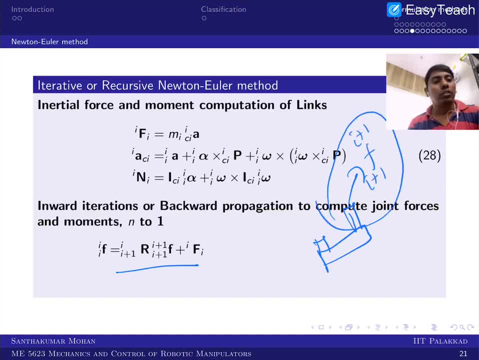 plus 1 to i plus 1, there is a individual force. okay, and as well as what happened, this is having a link force which is due to inertia. so now what i wanted, i wanted this f i to i, so what i can do this is actually like in i plus 1, that i can actually like backward to this, then i multiply. 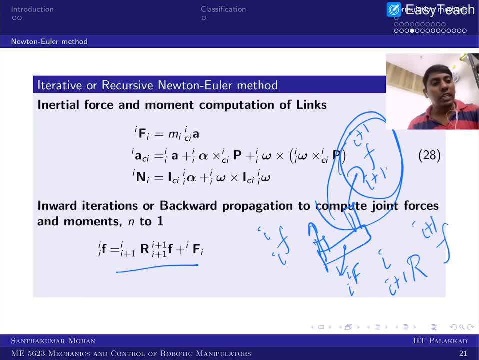 r i to i plus 1. so that is what i can see. this is going to come with respect to the i plus 1 effect on i that i can do, and then what i can see. i have one link which is having the link force also there. so now this. 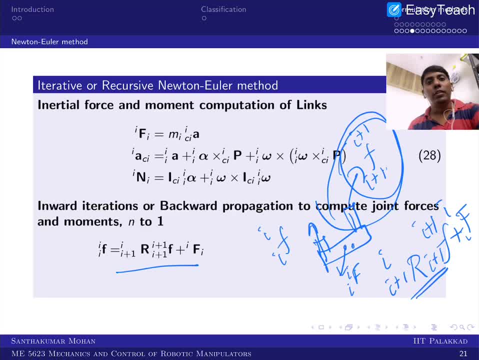 need not to be even linked. for, for example, i have a cable. so i have a cable which is actually like attached, the tension also. i can write: so now this is a tension force, okay, so like that i can add. then i can write that tension force of i right, like that i can keep adding. this is the advantage. 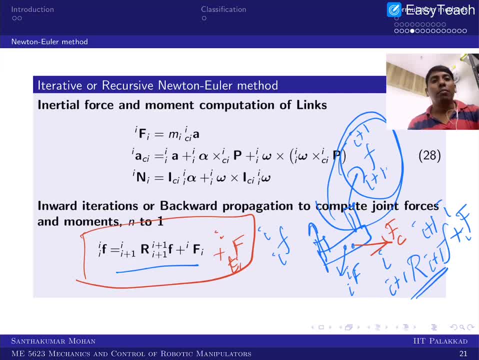 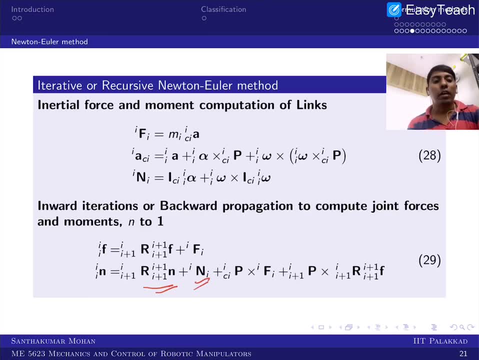 of having you call so called newton euler method. similarly, you can actually like extend the moment, so that means you can say the previous moment and the current initial moment will come. apart from that, your initial force also like trying to give what so called. you can say the moment and as well. 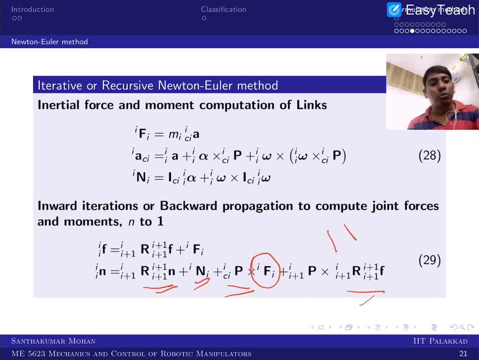 as your force for that, what i am trying to do, i am just trying to do so, something like this: okay, so now this is a centroidal- you can say force and this is a centroidal moment. okay, and here i am getting n. i plus 1. 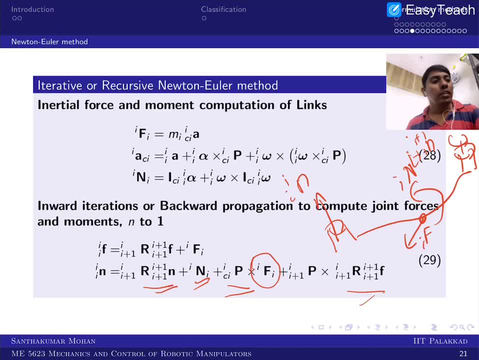 1 frame. I am actually like interested to find this. so what else would be there? so there would be actually like force also would be acting. so that is f- i plus 1 to i plus 1. so this distance I call p- i to i plus 1, and this distance I call p c i to i. okay, so now this actually like going. 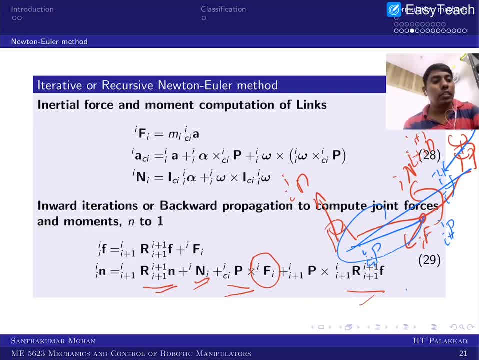 to give a couple f i into this. so in the sense r cross f. so here r is actually like p? i to c and this is actually like r cross f. this is actually like p? i to i plus 1 into f i plus 1. so these are the couple due to the force, and this is the initial moment and this is the 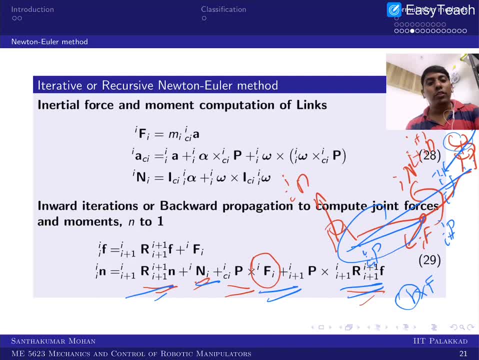 moment, at the point, or the joint n plus 1, that is, you are transferring here. so now, these two equations you know and you can actually like start from the- you can say- final joint, where the free joint, and then you can come backward, so just to give that finally what you will get. 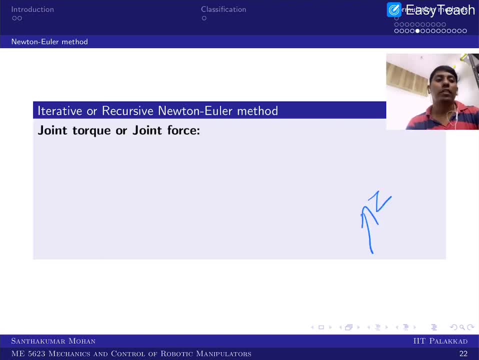 so you know, like every joint axis associated with that axis, if it is a rotary joint that is associated with the torque and if it is actually like a translation joint that is associated with the f, so that f would be the, you can say the final, whatever the joint. the third: 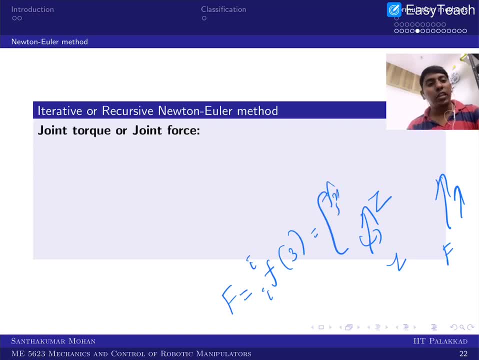 component. in the sense this third component is in the effects fy, fz. the fz would be corresponding to that particular joint force, right? so similarly, the joint arc you can see that is n, i plus or i, so that would be having n, x, n, y and n, z, the last joint, or you can say the last component. 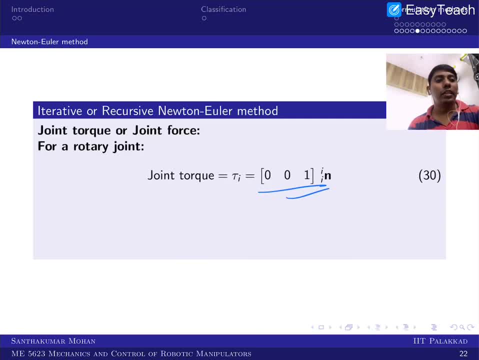 is related to the joint force. that is what we are trying to write here. you can see that I am actually like multiplying this. you call row vector. with respect to this column vector, you can see that the final component will come, so that is what you call torque vector. 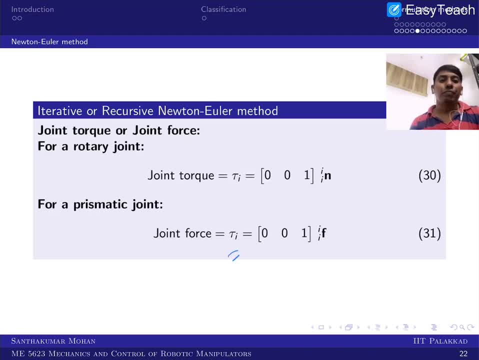 and this is what. sorry, torque, joint torque and this is the joint force. so we are trying to maintain single- you can say variable- for everything. so, tau, i is actually like either joint force or joint torque, so based on what joint we have. it is a rotary joint, it is a. 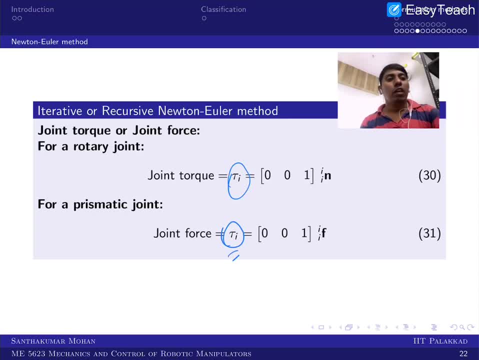 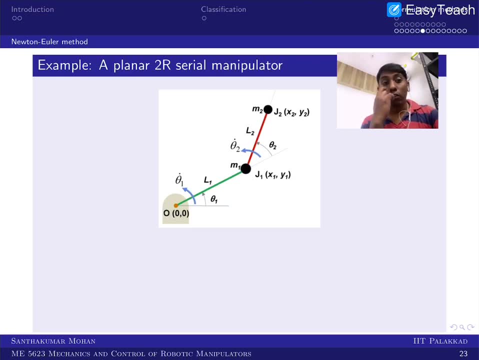 joint torque. if it is a prismatic joint, it is a joint force. now we will take a simple example. so the same example we can take and we will actually like, do the forward propagation for angular velocity and you can say linear velocity, then angular acceleration and linear. 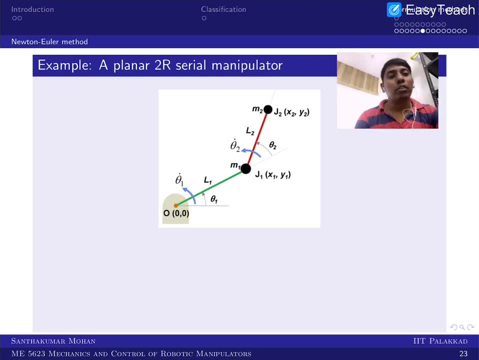 acceleration, then we will come back with the, you can say backward, while going itself we will find the inertial force and moment. so here actually you can see the centroid also like concentrated here, just to simplicity in the sense, what you can see, you can do the dh parameter and you can find the induced force. 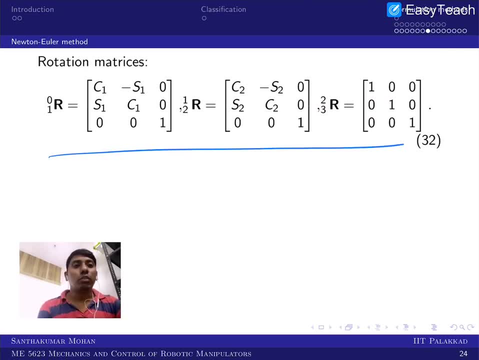 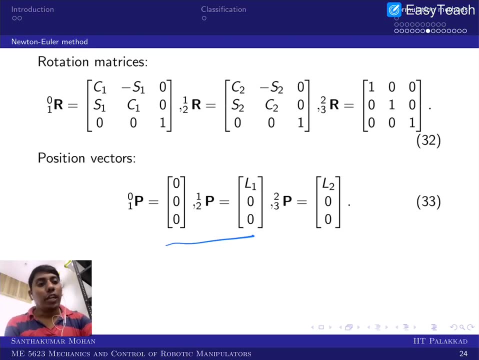 So here, individual, you call the transformation matrix, and then you can find the rotational matrix or rotation matrix, and then you can find the position vector. and now, when we are actually like doing the second thing, what you have, so P i to C i, so, for example, I am: 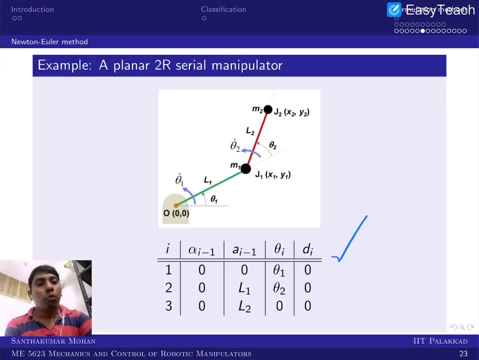 actually like trying to see here. so what would be the x i direction? so this is what. so I am just showing that. so this is the x 1 and this is what your first mass M, C1, 1 and you get the x 2.. 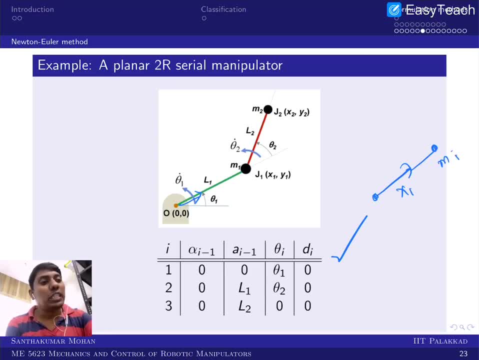 MC1 or M1 concentrated In the sense, what would be the CI? CI would be located here. So what would be the position of CI with respect to I? that is, on the x direction. that is actually like. the distance is L, So in the sense, L1, 0, 0 right. So now the second link you can see. this is what. 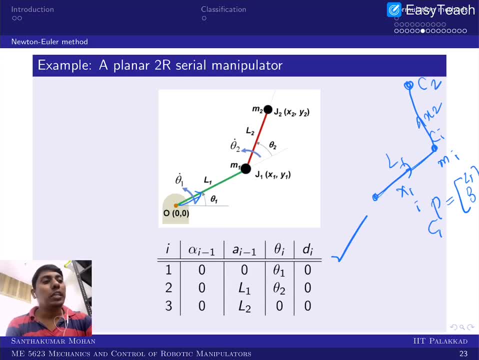 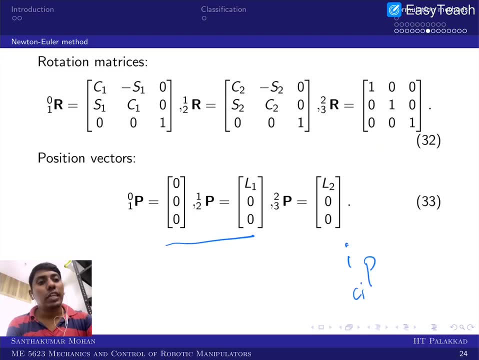 x2 direction and this is what C2.. So what would be the x2? or you can say PC2 with respect to C2, that is L2, 0, 0, right? So in the sense you can see that the position of centroid also, like we, 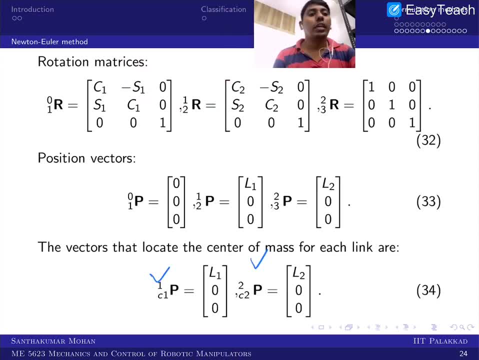 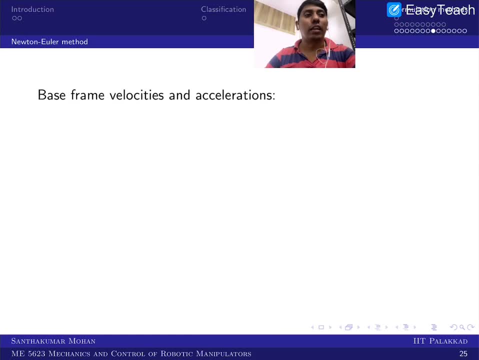 calculated. So that is what we are actually like doing it okay. So this is the position vector. come from the Dynavit Attenberg, but this is you have to physically calculate, in the sense you have to see and calculate. So once that is obtained, then you can go with the- you can say- base frame. 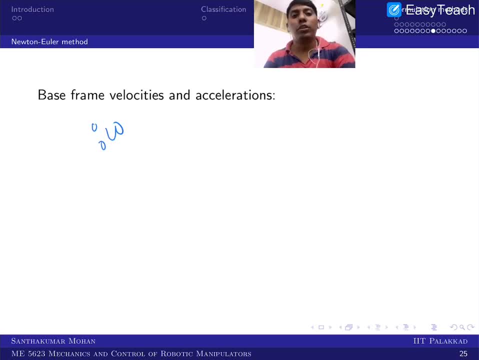 I assume that the base frame is fixed in the sense what happened? omega 0 to 0 is nothing but 0, 0, 0 and acceleration Also like zeros. in this case it is actually like 0 and y axis: there is a gravity and 0, y. 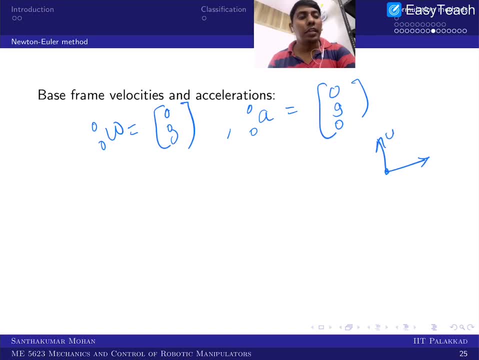 because we assume that this is x and this is y and this is z axis and your gravity vector is actually like in this case. So this is the gravity vector, So which is actually like I am writing, as you can see, g is actually like not this minus g, okay. So, in the sense, what I can try to see, 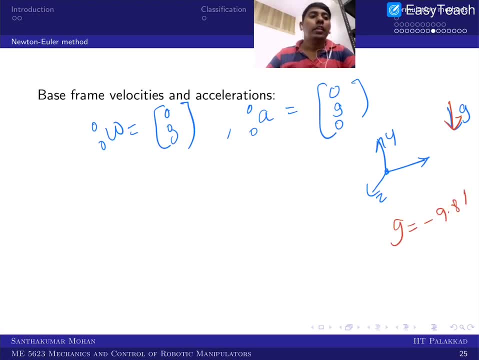 the g is, I will substitute minus 9.81. okay, So that is what. in the sense, what would be the acceleration vector? linear acceleration vector at 0 point. So the acceleration would be here. So in the sense, you can see the 0, g and 0. that is what. 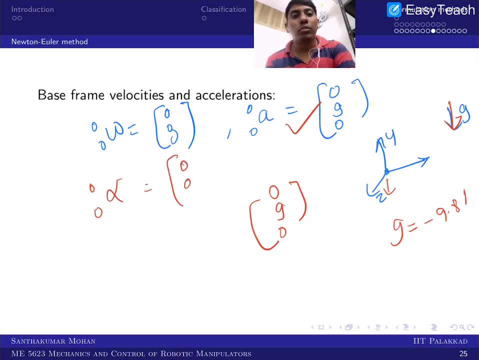 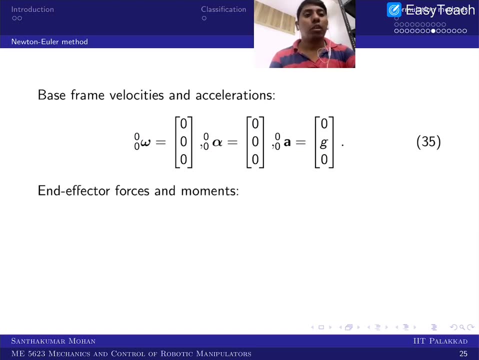 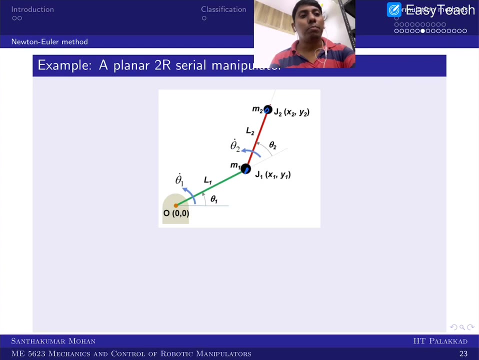 we can. So, similarly, alpha 0, 0 would be again 0 0, 0. okay, So this is what we are actually like. taking as a base frame velocity in acceleration, we can go forward, So what that means. so you are actually like seeing the end effector force. So I am actually taking here, you can see. so I have taken this point. 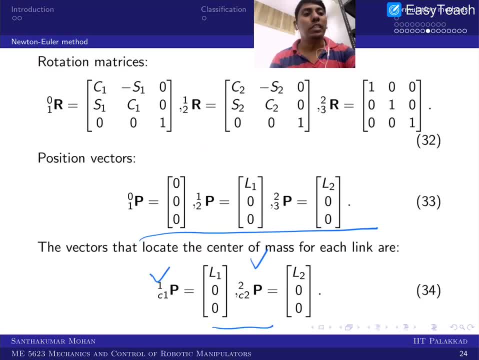 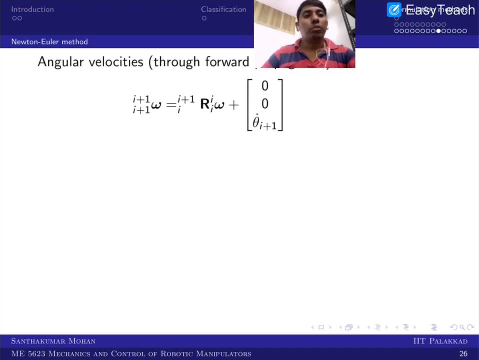 so in the sense end effector forces, where you call f 3, 3 would be 0 and n 3, 3 also like 0, just for simplicity. okay. So then what you can see. you know already the angular velocity propagation, you know already omega 0, 0, and you know r 1 to 0, and you know theta 1 dot also there. So then what you can: 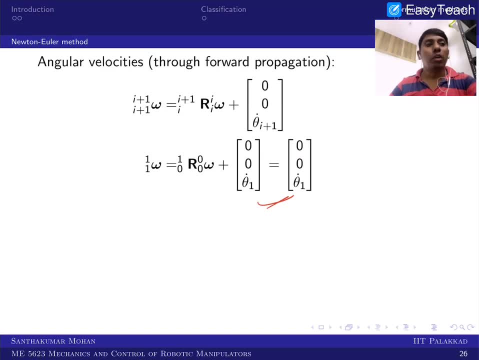 see, you can actually like propagate this. So then, omega 1, 1 known then omega 2, with respect to 2 also, you can calculate the same way and you got it Similarly, you go 3.. So then, what you can do, you can actually like go acceleration, So angular acceleration, you can start. 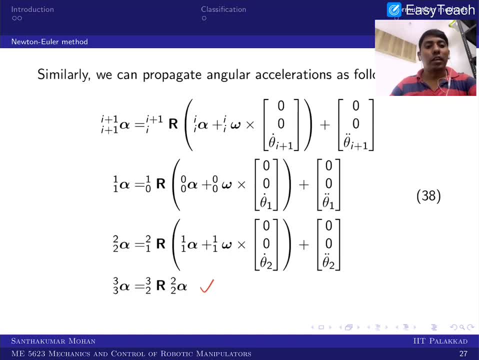 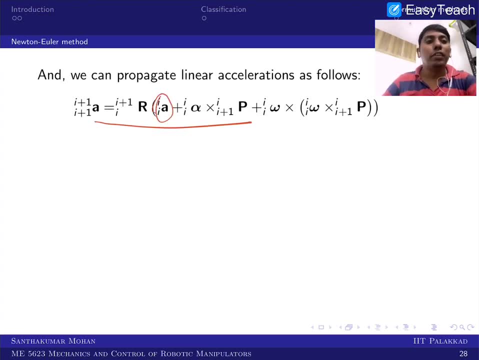 with the same way and you can actually like see that these are actual, like uptime, right. So now, what you can do now you can go with the linear acceleration, the linear acceleration previous and the- you can say that, you can say tangential- and the radial component. you know, because here 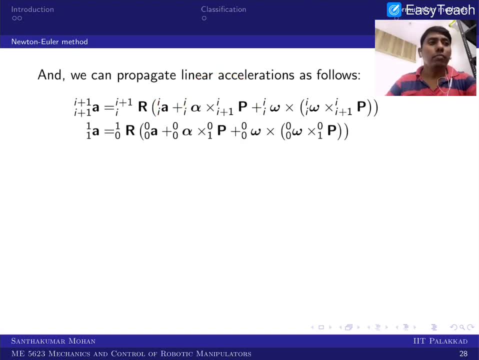 everything is row t, So you can actually like find it So: a 1 with respect to 1, we calculate, and a 2 with respect to 2, also calculate. a with respect to 3, we can calculate. So now, what you can need to calculate, you need to calculate the centroid. 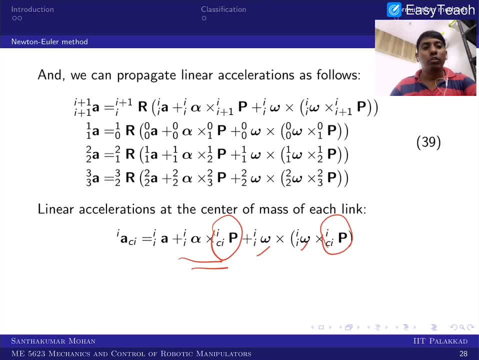 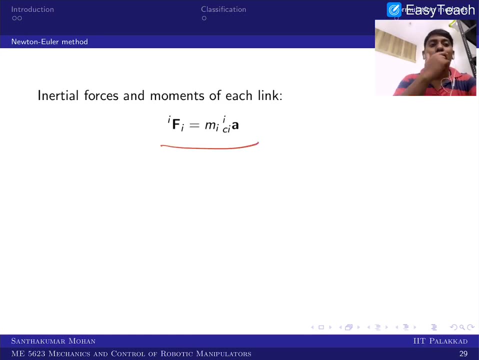 So here this vector is known and what you know- these are individual joint velocities and joint acceleration- is known. So you can go further, so you can calculate acceleration at point. you can say, the centroidal 1 you can calculate. So now you can see that these two calculated. then what you can calculate, you can calculate. 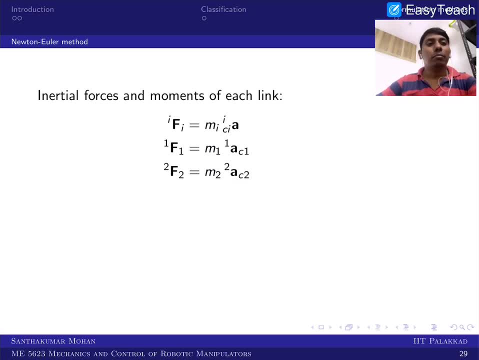 the initial force and initial moment. In this case, initial moment would be 0, because we assume that mass is concentrated at one point. So then you can see that I would be 0, then you can see N1 and N2 is 0.. 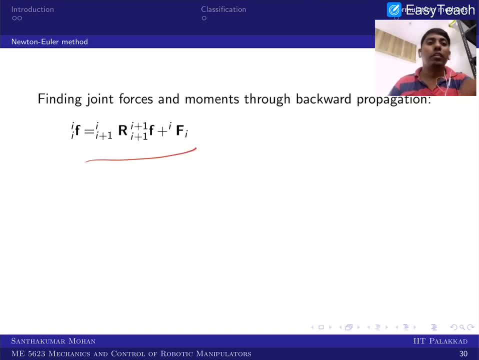 So in the sense F1 and F2 only there. so you can substitute that in the backward propagation where we start with the F3, 3 is known and F2, 2 is actually, like your link, initial forces, that is known. then you can come backward. 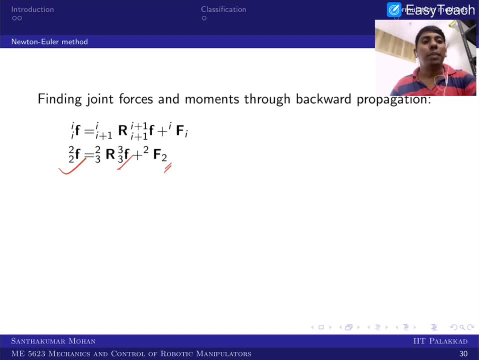 So what? you can see, that F2, 2 is obtained and based on the n equation, you can actually like find the moment. So now the F1 and F2 also I calculated, then I will come back with n. where the moment? the moment you can see that this is there. 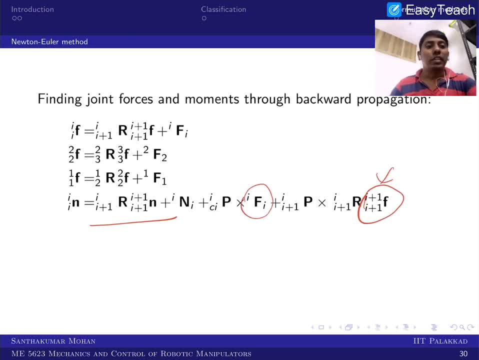 So in the initial joint, this is going to be 0, but you can see this is there and this is are existing right, So, and this is obviously 0 and there is no moment also in this case. So then, what you can see, you can actually like get these all and you can actually like. 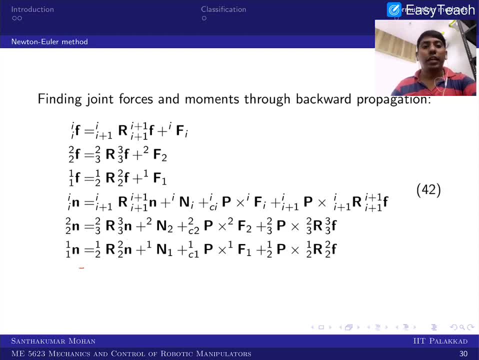 still go forward, sorry, backward. and then you can find n1. So if you want to know what would be your, you can say base forces And base moment. then you can come backward till this. but right now we are interested in to find only the motion dynamics, the sense equation of motion. I can stop up to the active. 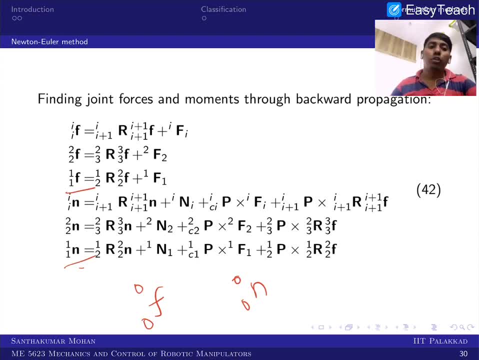 joint, which is 1 right. So that is why I stopped here. if you want to know the base forces and moments in the sense what we call shaking forces and moments you want, So then you can go, then you can see what would be the support, reaction and moment, and then